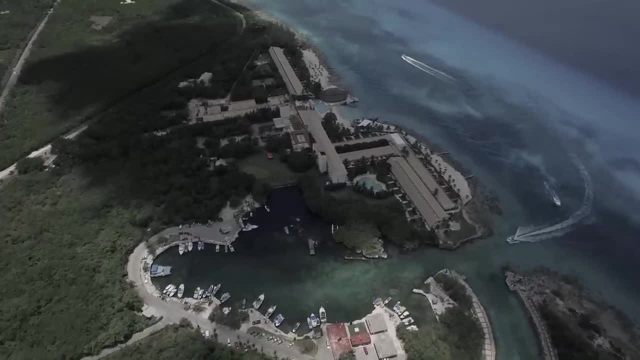 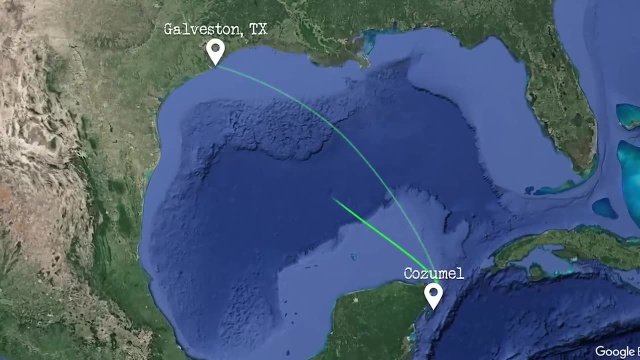 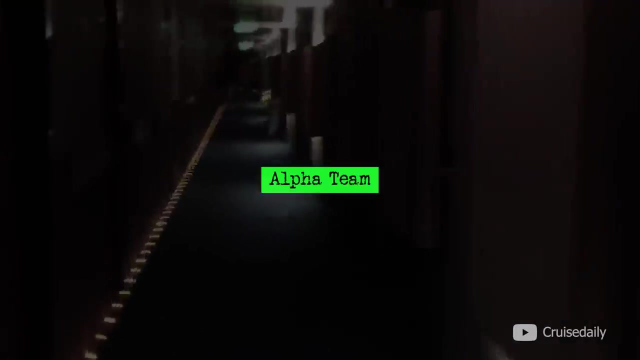 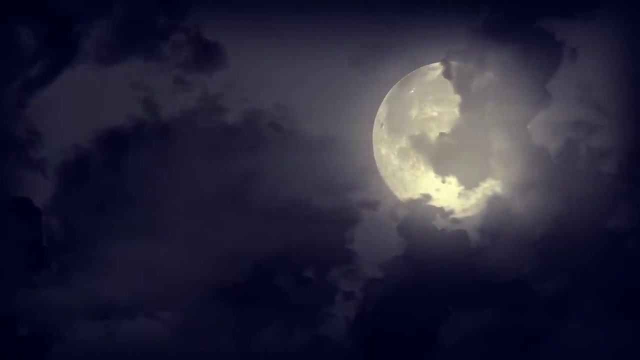 frolic in azure waters, shop to their hearts delight and return for a night of festive on board activities. in reality, after departing cozumel for the return trip to galveston, the crews took a turn for the worse. in the early hours of sunday, february 10th, a fire alarm echoed through the ship with the alpha team. 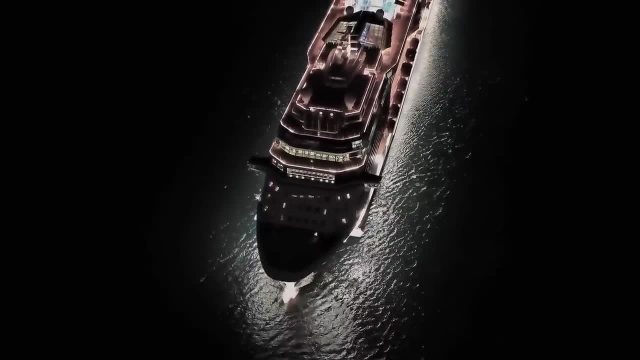 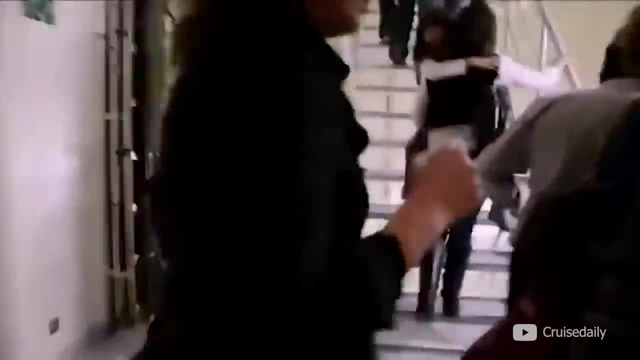 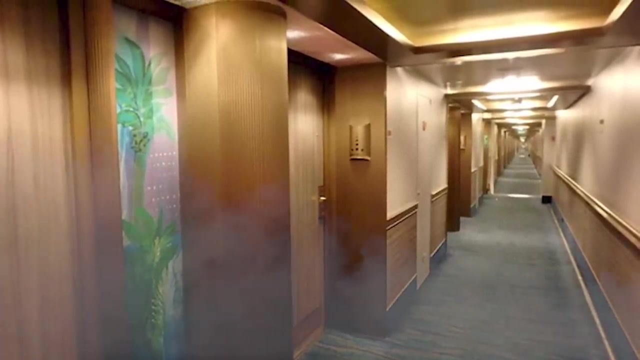 call booming over the pa system shortly after 5: 28 am, the alpha team announcement- the code used for a fire emergency aboard carnival vessels- left many holiday makers panicked. guests on the first and second decks opened their doors to find smoke-filled hallways. chaos broke out with 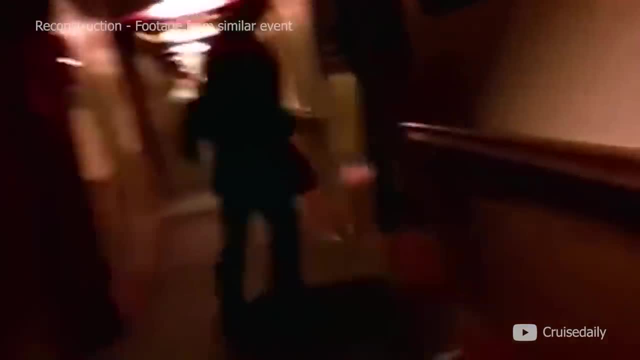 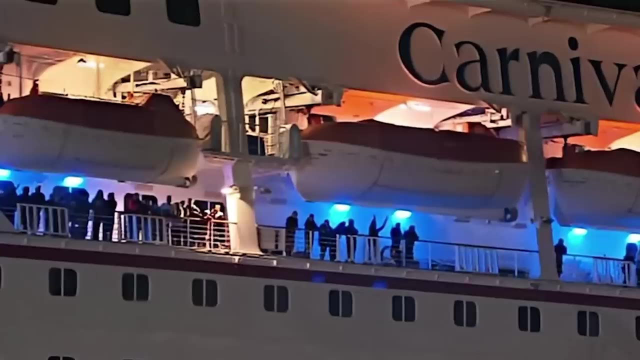 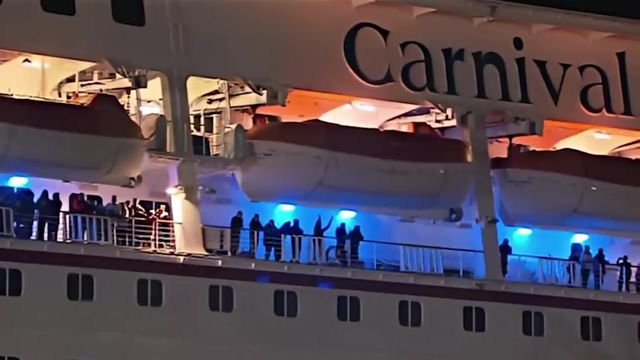 passengers scrambling for life jackets and frantically searching for friends and loved ones. on the top deck, black smoke was billowing from the smokestack. the alpha team alert led to panic among passengers, with some heading to evacuation stations once they heard no further information or instructions, while the announcements called for calm. 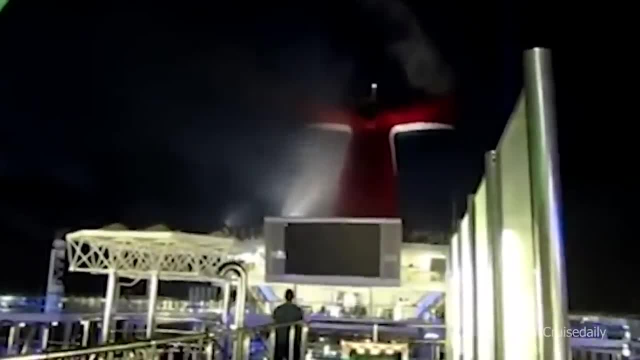 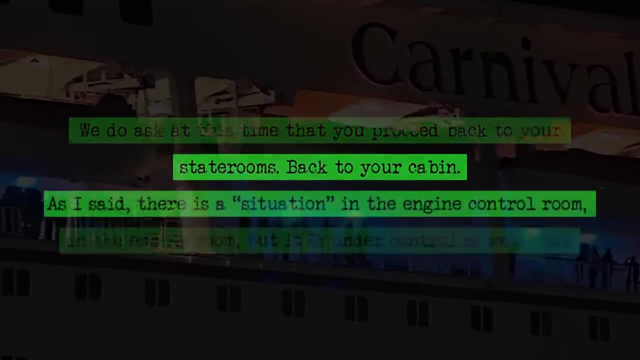 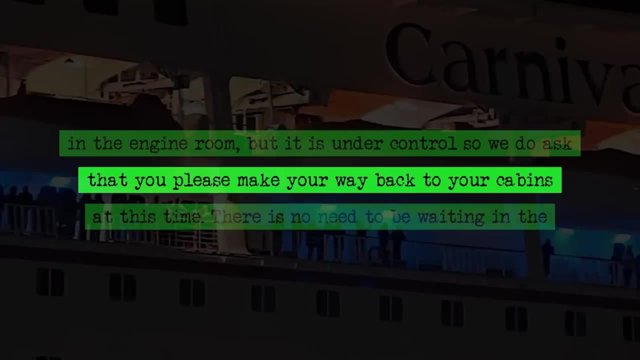 guests were left in the dark about the extent of the fire. folks, there's no need to be at the muster stations. we do ask at this time that you do proceed back to your safe rooms. as i say, there is a situation in the engine control room, in the engine room, but it is under control. so we do ask that you please make your way back to your 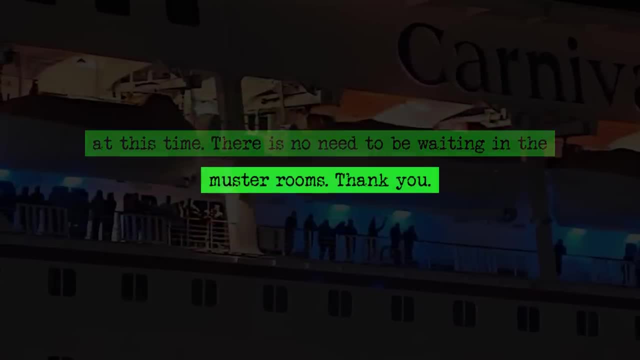 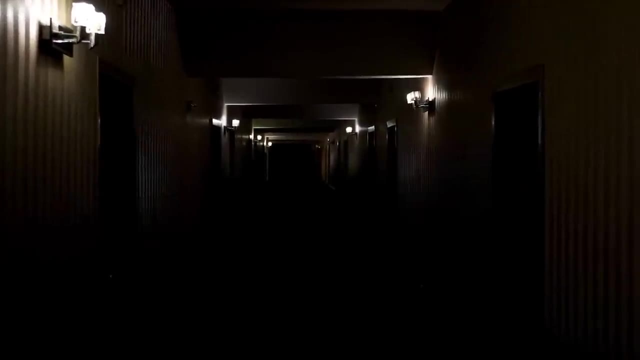 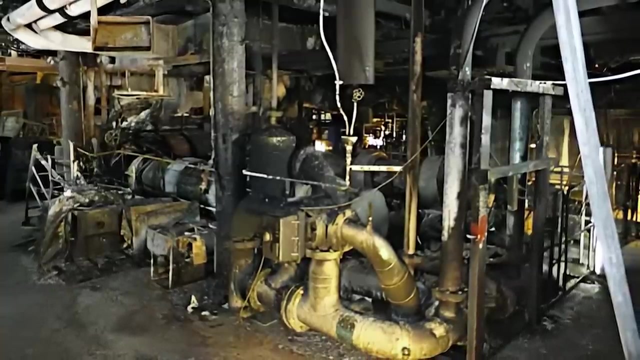 cabins. at this time, there's no need to be waiting in the muster stations. thank you. soon after the initial announcement, the ship's lights flickered before it lost all power, except for the emergency lights. the blaze, which was contained in the engine room through an automatic fire suppression system. 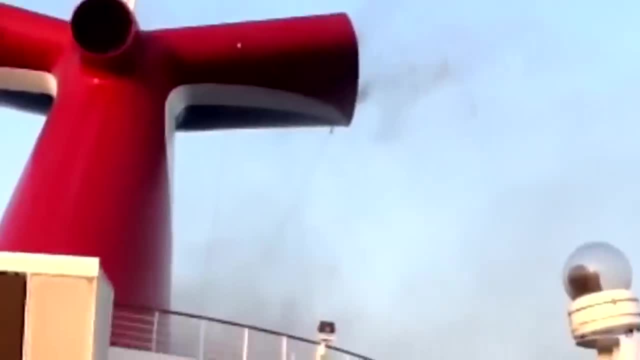 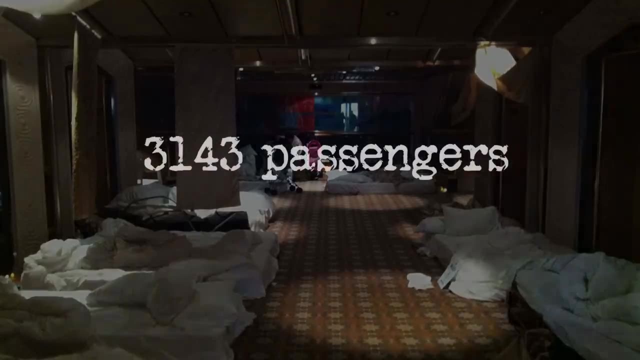 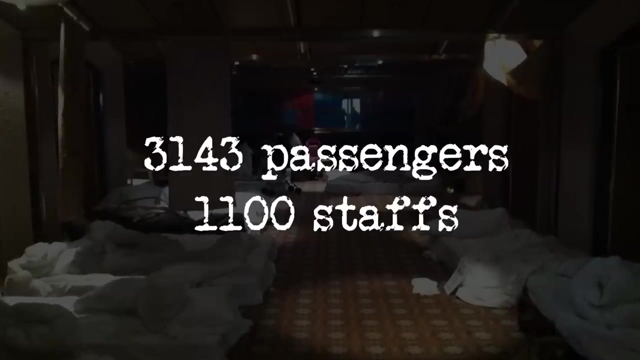 was reportedly quelled by 608 am. unfortunately, the fire had knocked out most of the ship's power and disabled the propulsion system, leaving the 3143 passengers and close to 1100 staff stranded in the gulf of mexico. but there was a plan: two tugboats set course for the stricken vessel to tow it to the nearest port. 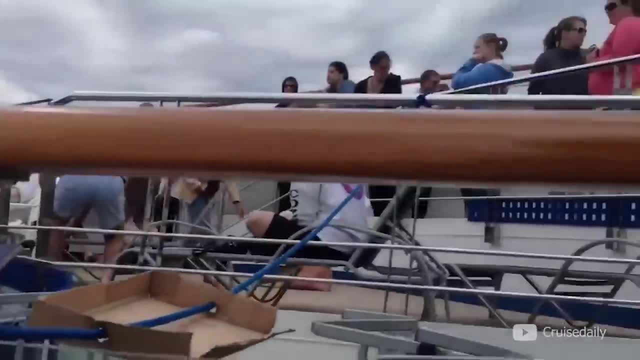 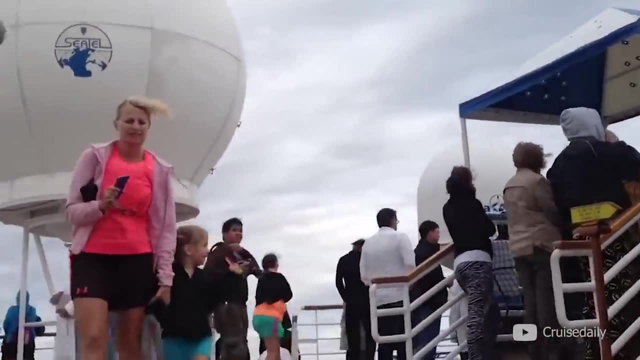 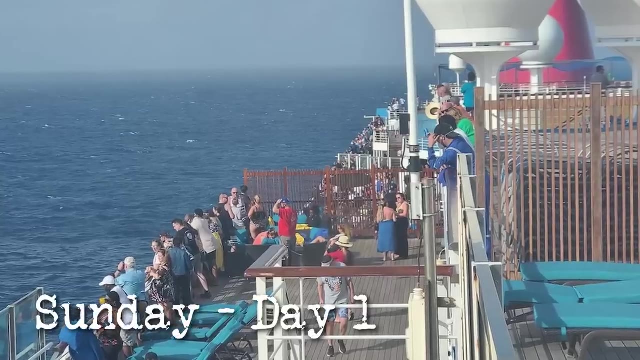 of progreso mexico, passengers breathed a sigh of relief and started taking off their life vests. docking by tuesday, they were told. little did they know another four days would pass before anyone set foot on land again. by mid-morning on sunday, passengers realized it wasn't just the propulsion system that died: the air conditioning. 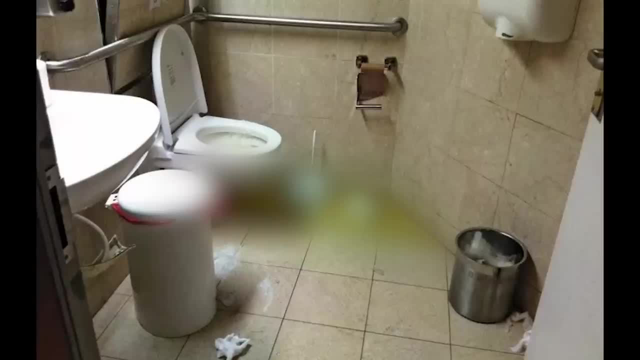 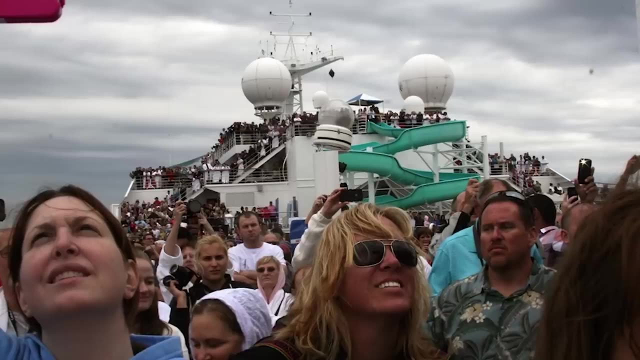 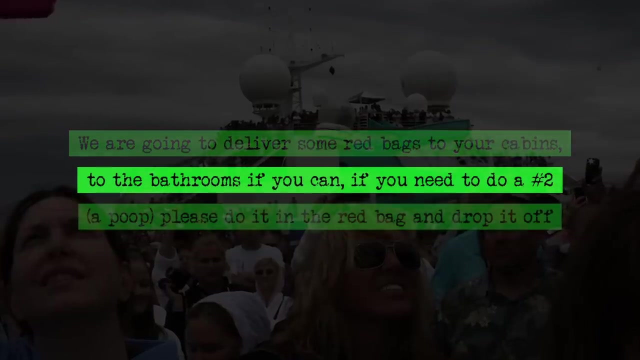 running water elevators and, worst of all, the septic system had also failed. that's when the cruise director delivered a message that left passengers horrified: we're going to deliver some red bags to your cabins, to the bathrooms, if you can, if you need to do. you know a number two: you need a poop. please do it in the red bag and drop it off in the bins in. 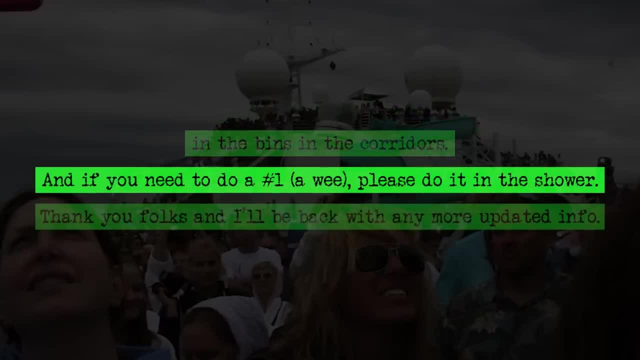 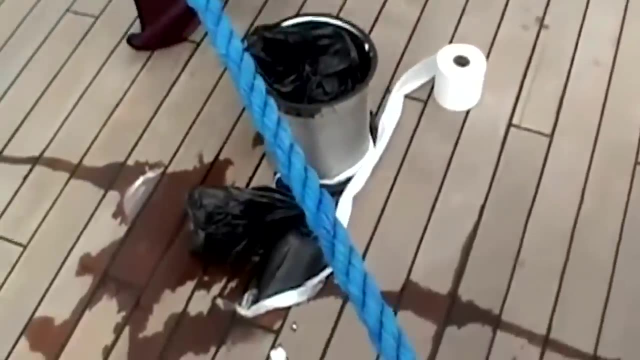 the corridors and if you need to do a number one- that's a wee- please do it in the shower. thank you, folks, and i'll be back with any more updates from the crew. this announcement came when toilets were already clogged due to lack of flushing facilities in the 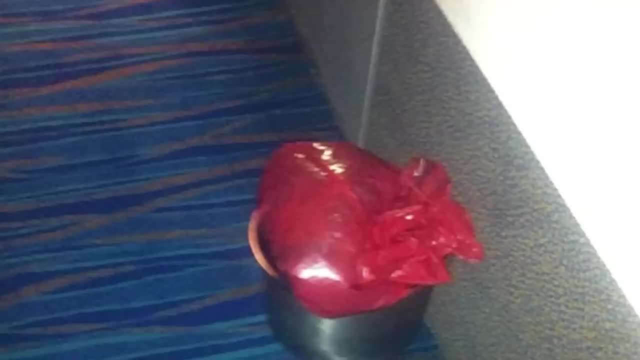 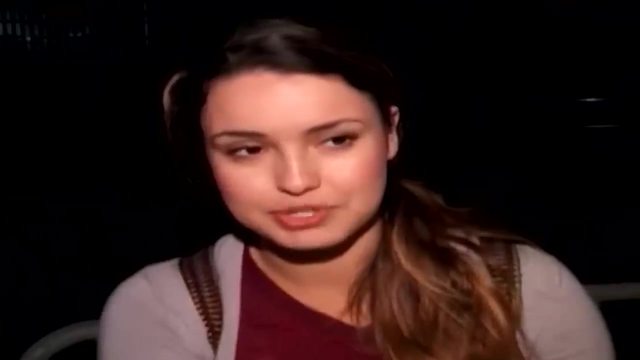 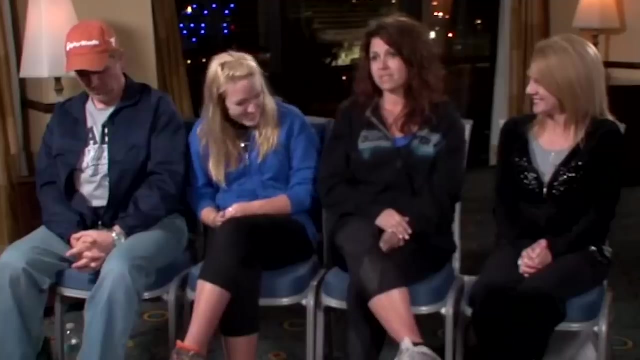 private cabins and public restrooms. the now infamous red poop bags were just too much to bear for many passengers. people were using the restroom in little red plastic bags and throwing them out into the hallway. we were in shock. we were like i'm not using a red bag. the thing is, 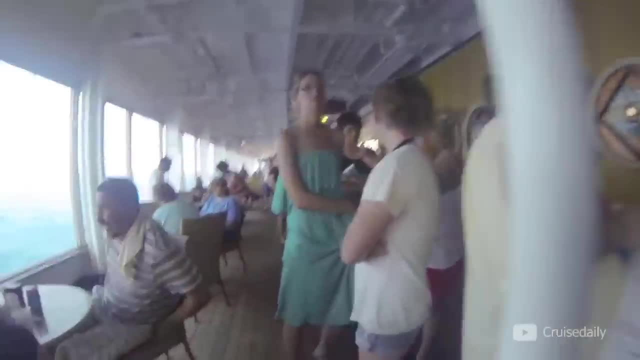 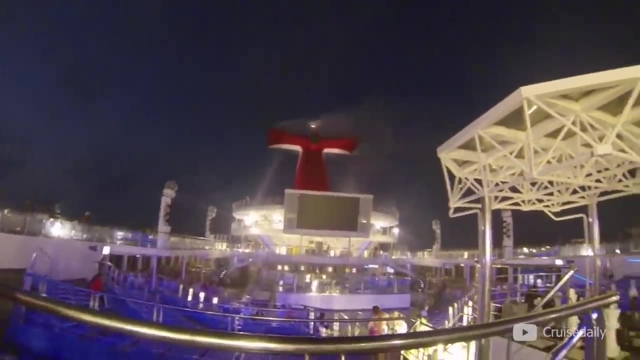 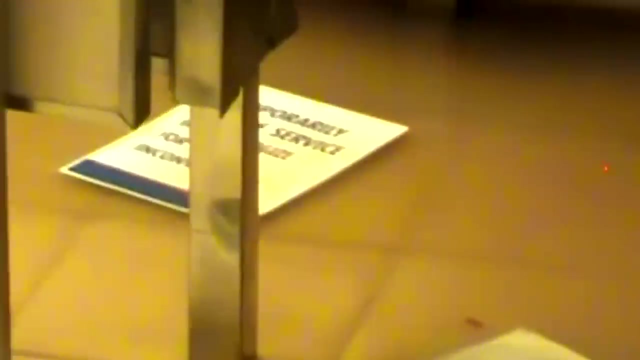 you just don't eat. the triumph stabilizers also took a hit from the fire, causing the vessel to list heavily. passengers reported clutching walls to keep their balance. but, worst of all, toilets overflowed and spilled into halls, seeping through walls to floors each time the ship tilted with the 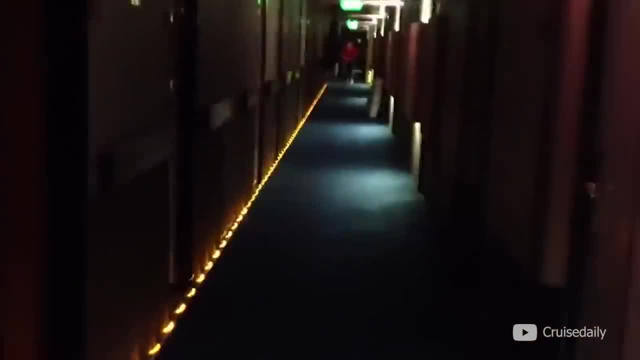 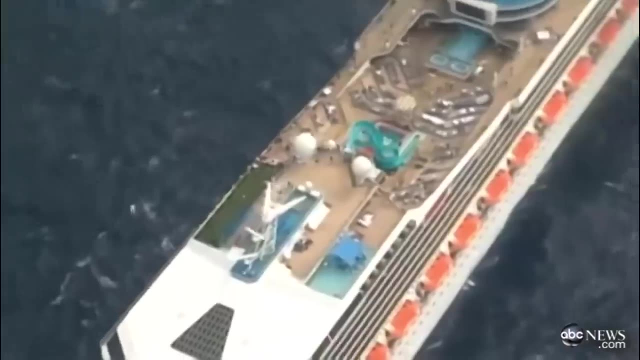 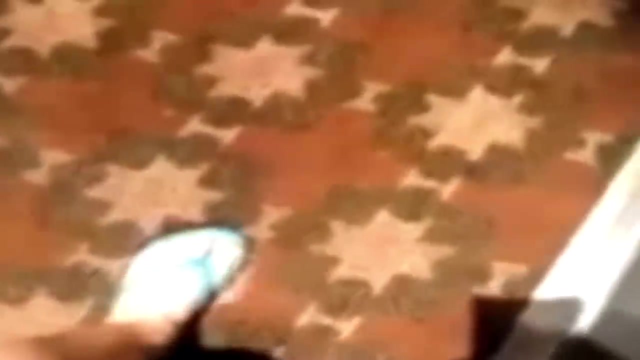 wind before long. images emerged of sewage, sodden carpets, bins lined with red bags and, in some cases, erupting toilets, depending on where the drains in the bathroom were. water and fecal matter came back up by the side of the bus and as we finished our visit, we were informed that there had been a 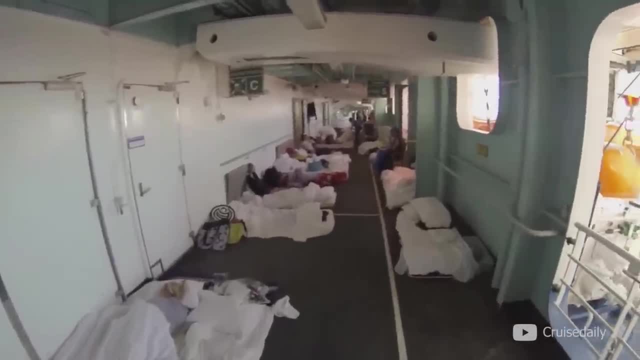 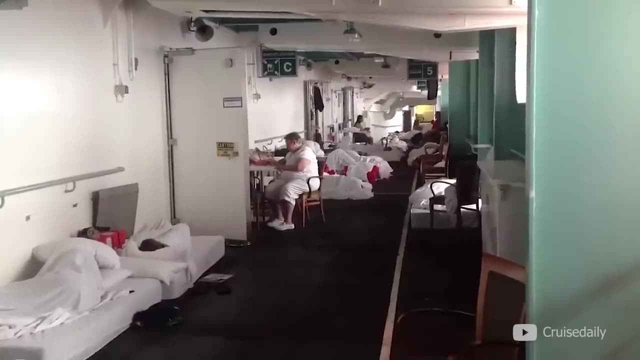 fire and that the stars and the sea water had spread across the back of the cabins. a lot of passengers were told and thousands were against the idea of making this a public circuit, but they were all aware of the cast and no one in the cabins believed these things. 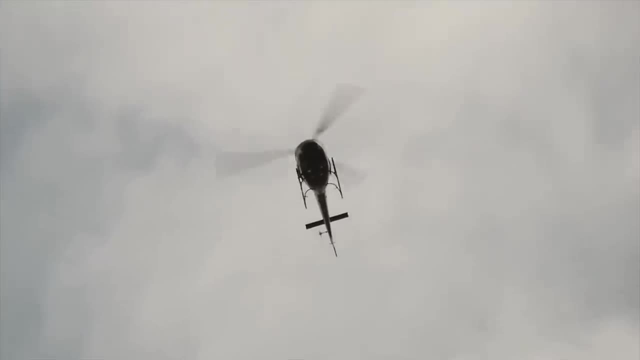 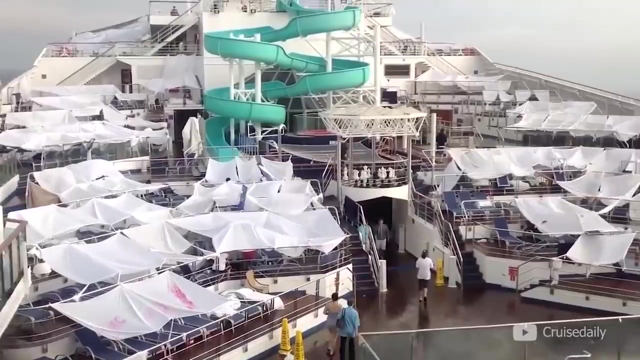 were actually real and they decided to leave the cabins to escape from the smell of the cold and the heat that was oppressing them along their beds and the passage to the cabins, with temperatures soaring in. the foul stench of human waste permeating the cabin, decks many guests. 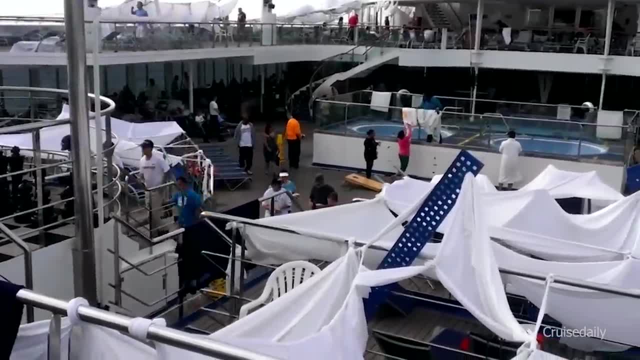 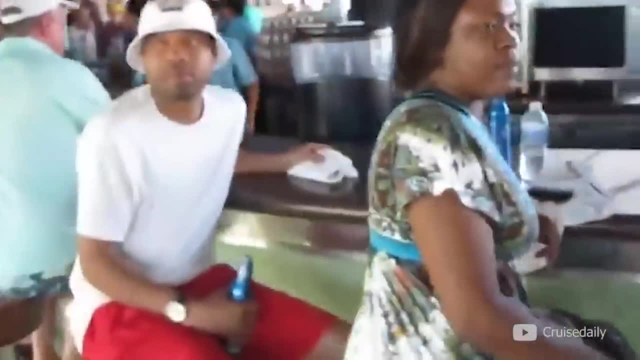 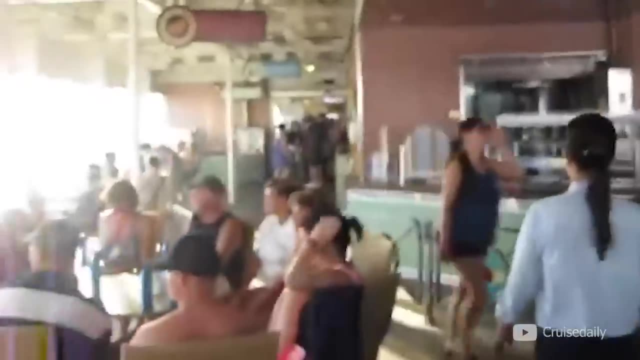 rope to construct makeshift accommodations on the tanning deck. In a bold attempt to quell the passengers' mounting frustrations, Carnival decided to host an open bar offering free beer and wine after the fire. The bar service was to run from afternoon until midnight, but turned out. 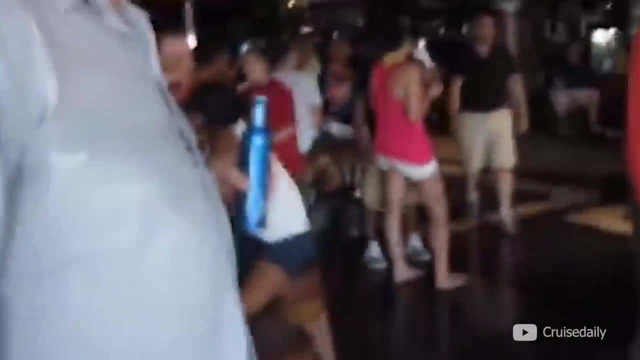 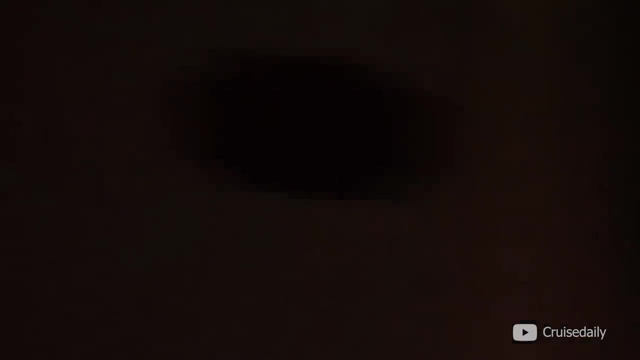 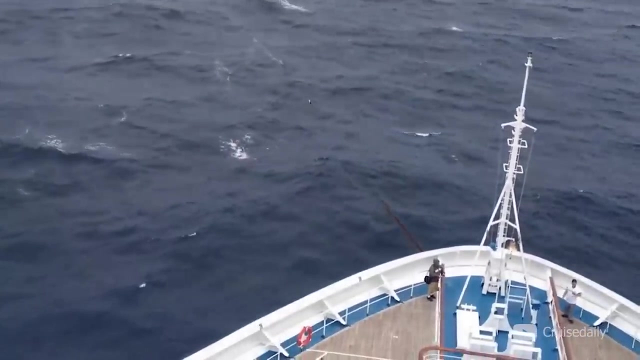 to be a terrible decision. With drinks flowing freely, several passengers became obnoxious and intoxicated, lobbing objects into the water and messing up the restrooms. By Tuesday morning, when both tugboats finally arrived, the vessel had drifted more than 90 miles north. meaning that Progreso was no longer the closest port. The decision was made to tow the 102,000 ton behemoth to Mobile Alabama, adding another two days to their journey. On the bright side, returning to the US would ease re-entry for the 900 passengers. 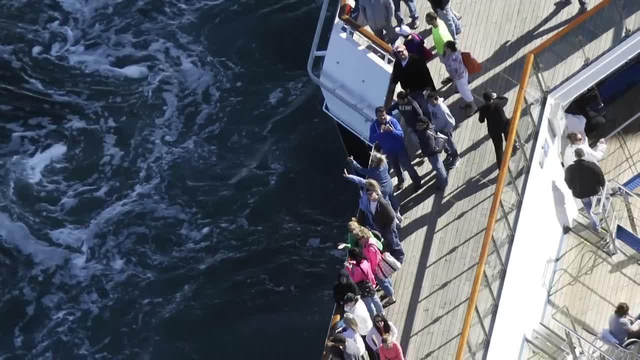 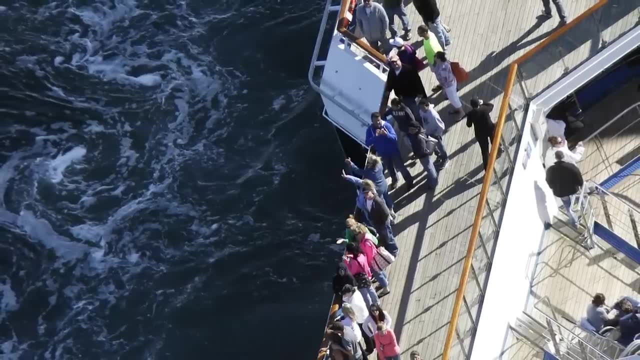 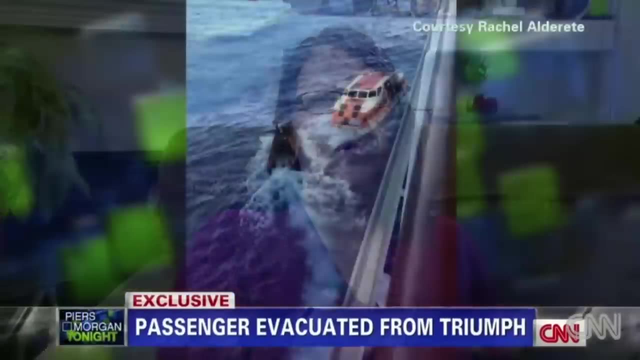 Traveling without passports. However, the added delay risked one passenger's life. Rachel Alderette, urgently requiring dialysis, became the first of only two people evacuated by the Coast Guard. They got the Coast Guards and transferred me to another boat, another ship. 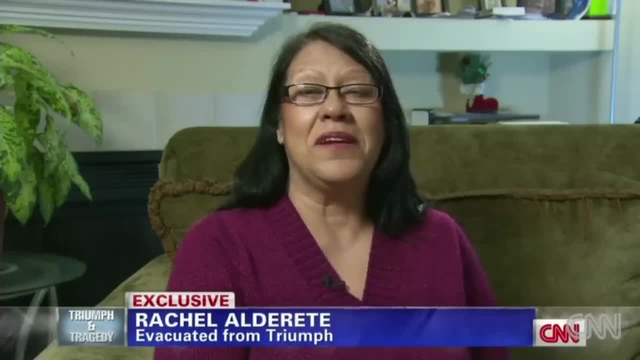 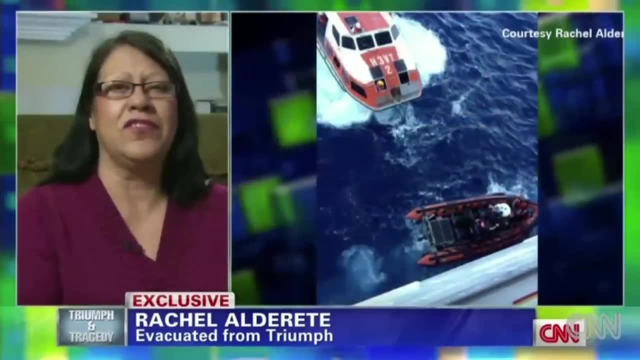 sent me to Cozumel to do dialysis on Tuesday. It was hard, It was scary, It was- oh my God, you know it was just scary the way they put me down. They put me in a stair rope and the Coast Guard said that don't worry about it, that they would. 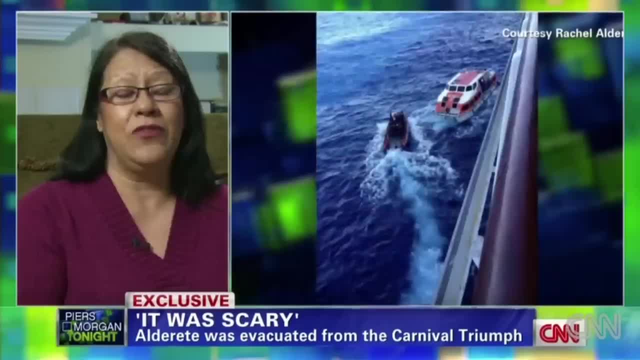 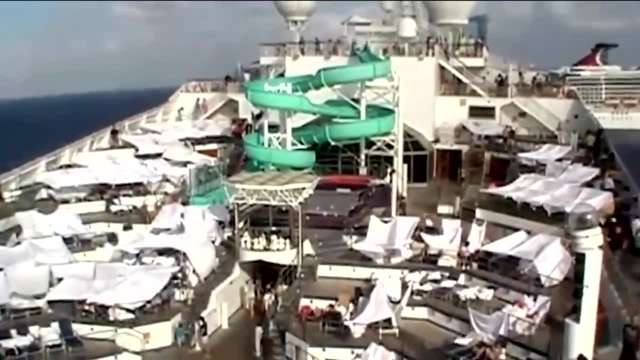 catch me and you know they were going to hold me back and they did, And then they transferred me to the bigger boat and, you know, The following day a second passenger was taken off the ship because of a pre-existing medical condition. Both were moved to other Carnival. 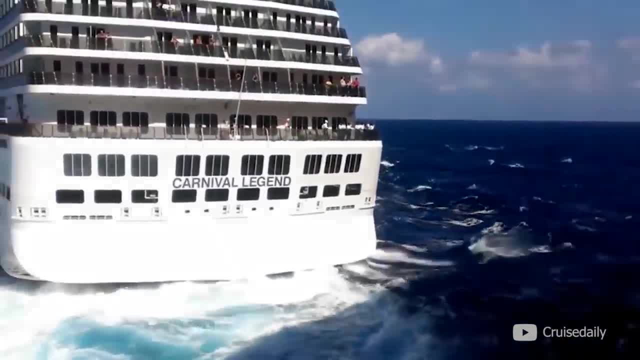 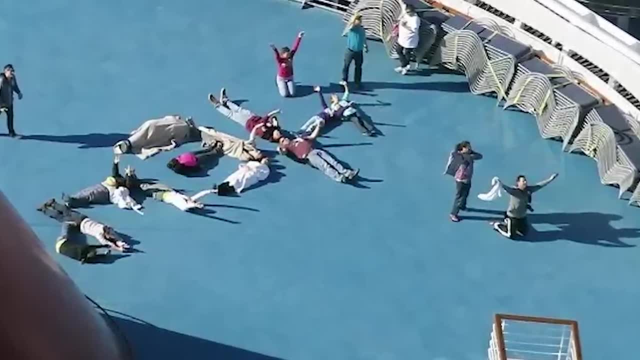 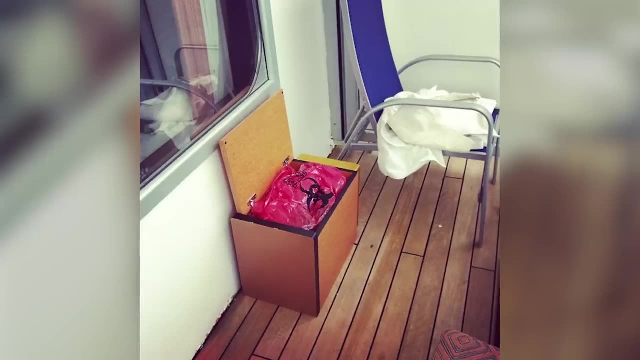 ships that had diverted their courses to assist with the rescue mission. Passengers commended the crew for doing everything they could To meet the traveler's needs, but that the toilet situation had been trying at best. Now that is. the problem with the boat is that the toilets have not worked and they 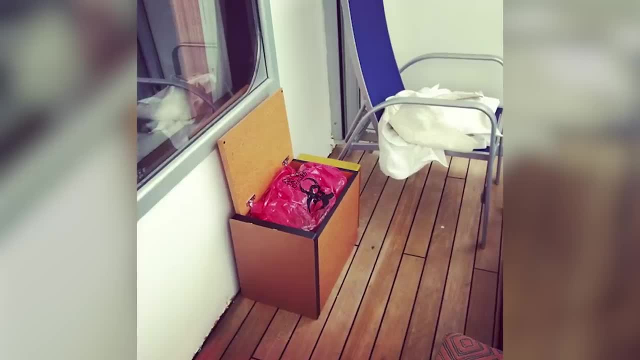 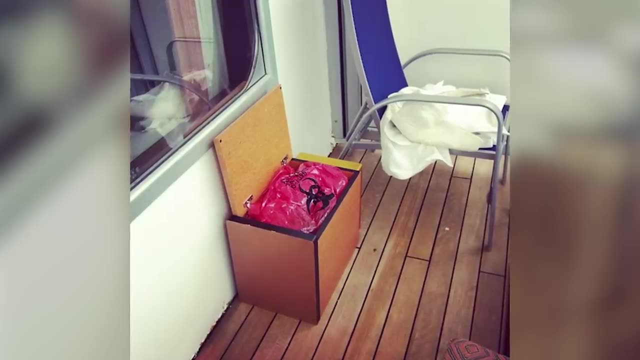 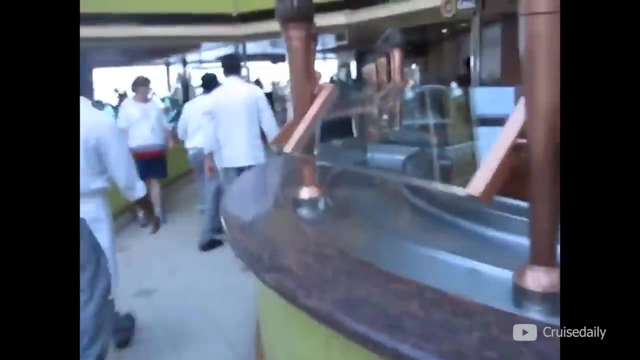 ended up having to issue us these bio. we call them the red bags, And that is what's been used almost exclusively for the first two days after the fire. Conditions on board rapidly deteriorated during that time and food was reportedly running out. Dwindling food supply was not the only problem. 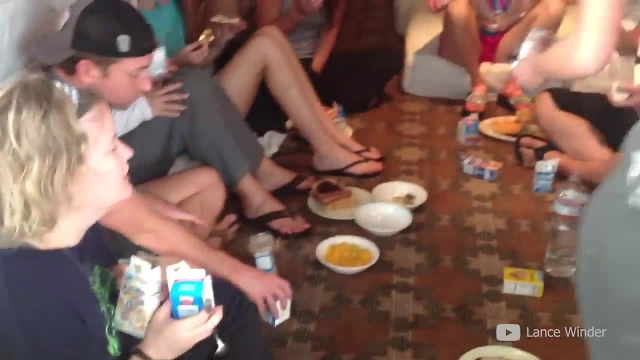 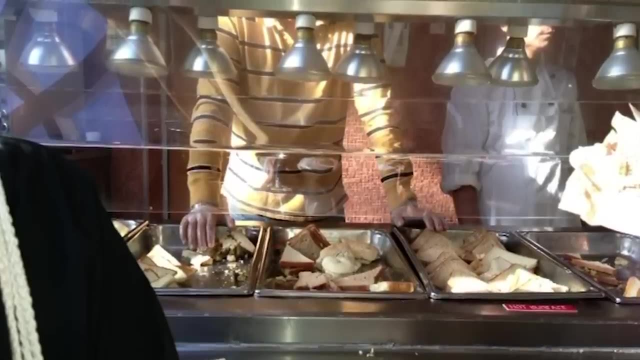 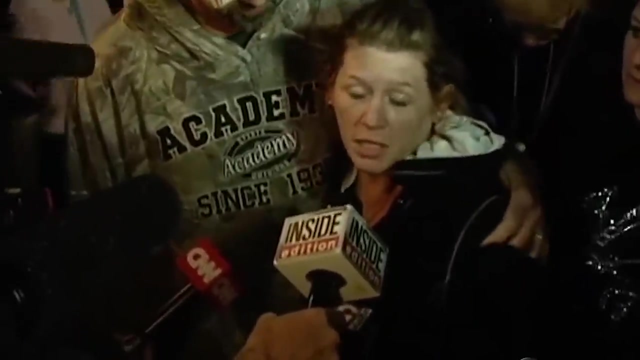 Food supplies forced passengers to queue for hours for cold onion and cucumber sandwiches. One passenger described scenes reminiscent of the Hunger Games, as fights erupted over dwindling provisions And they would gripe at you or other people would practically cuss you out because you would have multiples that you're trying to get for your whole cabin. So everybody wasn't. 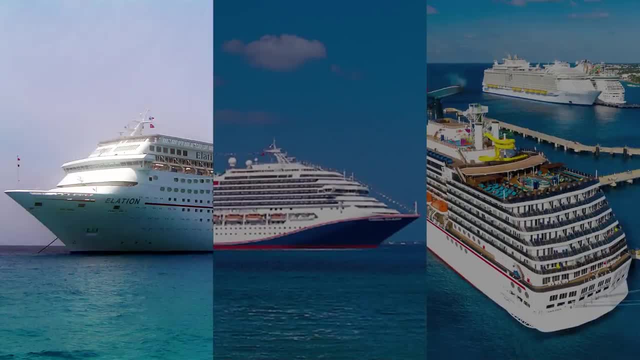 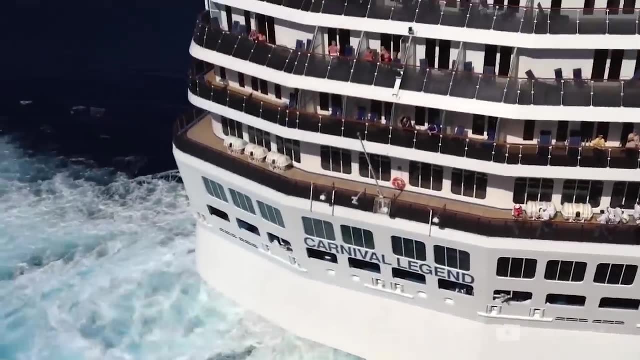 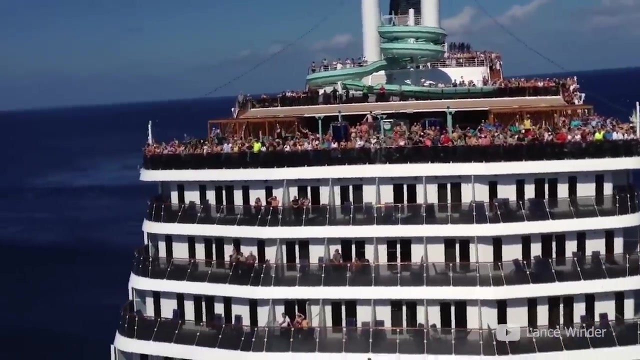 standing in line, Three other Carnival liners- Elation, Conquest and Legend- performed impressively. They were the only ones that were able to keep up with the pace of the ship, The tugboats clearly lacking the muscle to pull a ship of Triumph's size adequately. 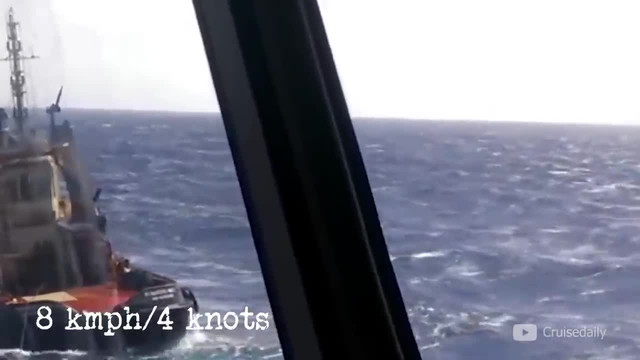 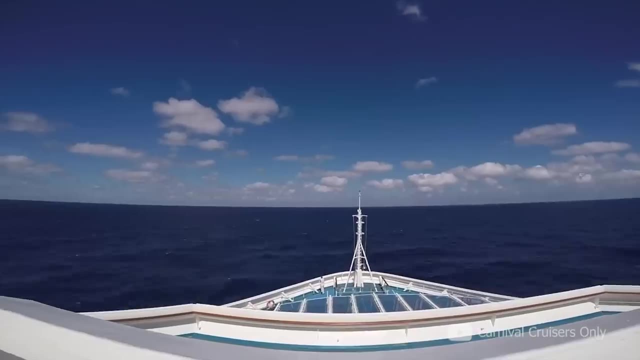 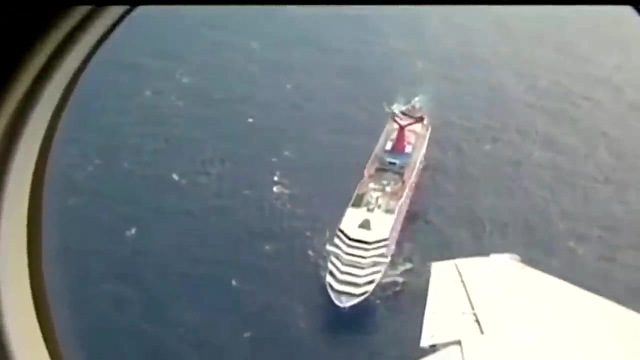 only managed a leisurely pace of about five miles per hour. Naturally, it didn't help that the tow line snapped several times during the process. Major news networks reported on Triumph's arduous journey to Mobile, with around-the-clock coverage of the so-called 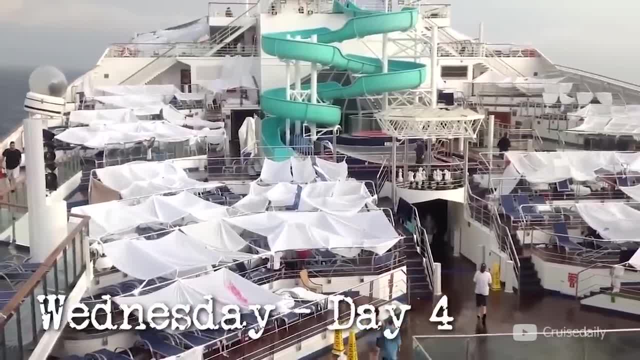 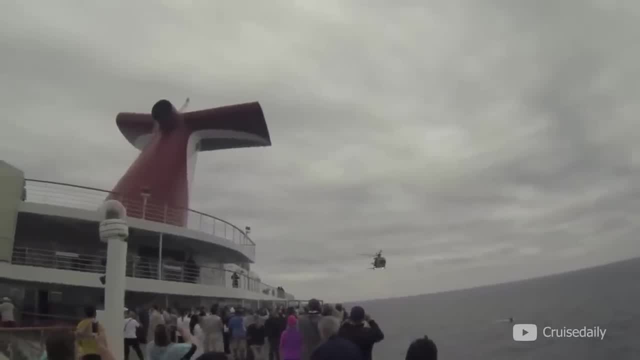 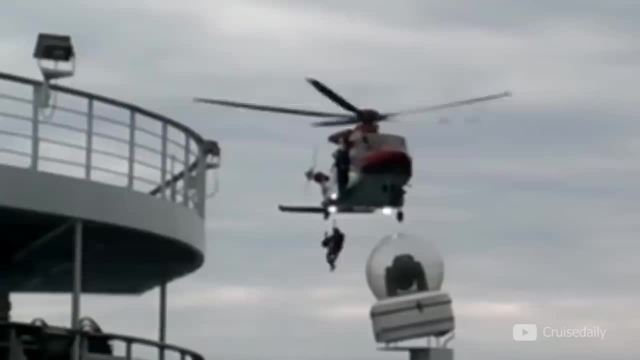 floating petri dish. On Wednesday, February 13th, Tent City had to be dismantled to make way for an incoming chopper delivering much-needed supplies and equipment. By Thursday, the mood aboard seemed to get a little lighter after the food drop and the arrival of a generator that promised 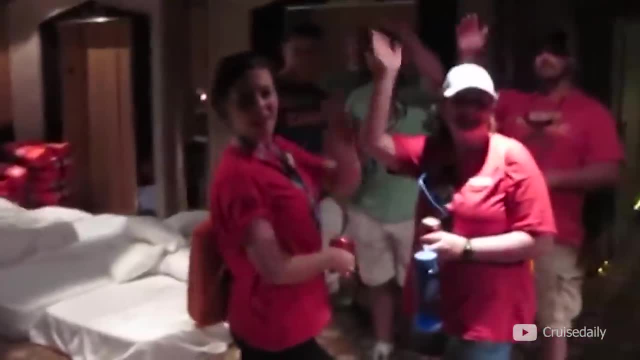 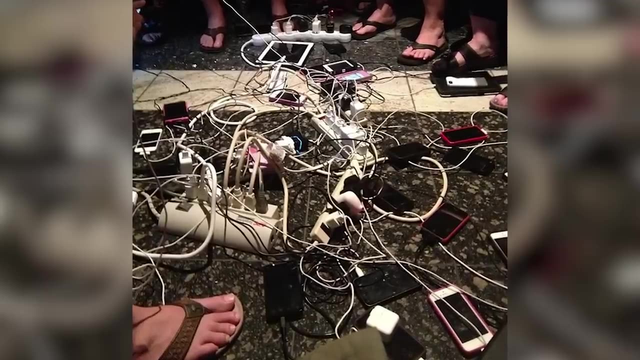 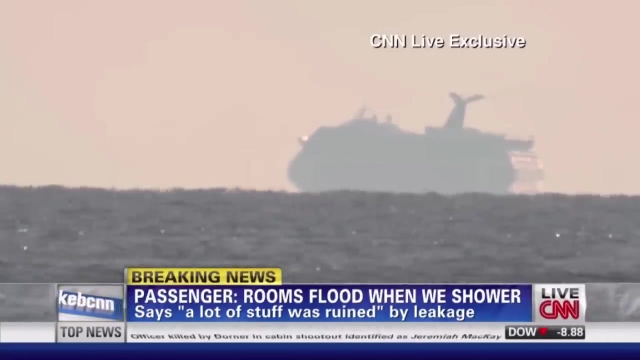 the luxury of hot meals. By this time, sanitary facilities were restored to parts of the ship and passengers had access to power outlets to charge their cell phones. For many passengers, staying in contact with loved ones had been a battle. We've spent the past two days about four to five hours a day charging our phones, so 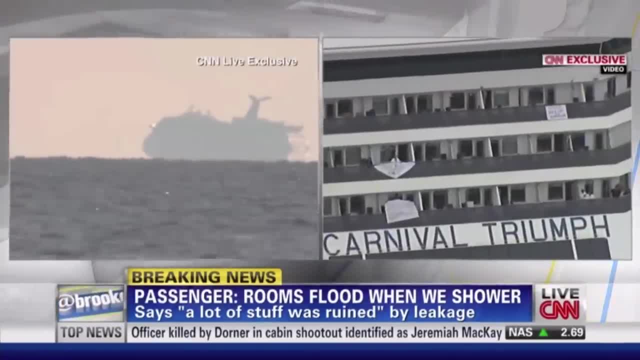 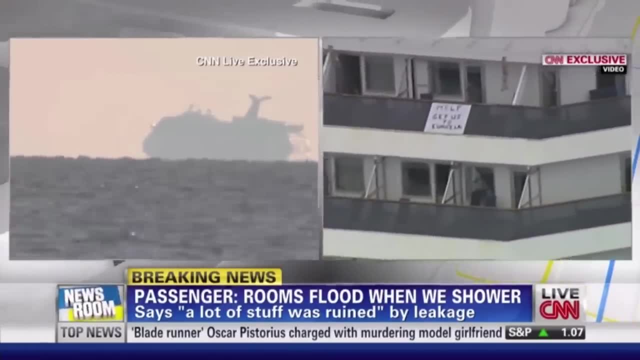 we can at least have the opportunity to talk. The only time we get cell reception is if one of the other cruise ships comes close enough to us. So we've all been frantically charging and we've actually rigged charging stations from ship computers to try to get. 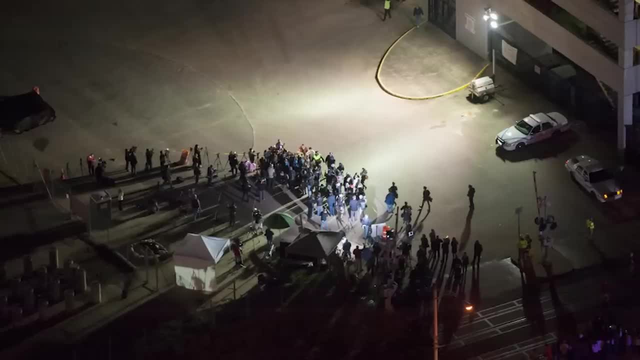 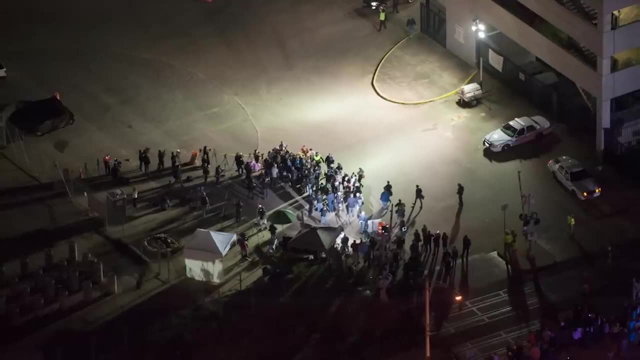 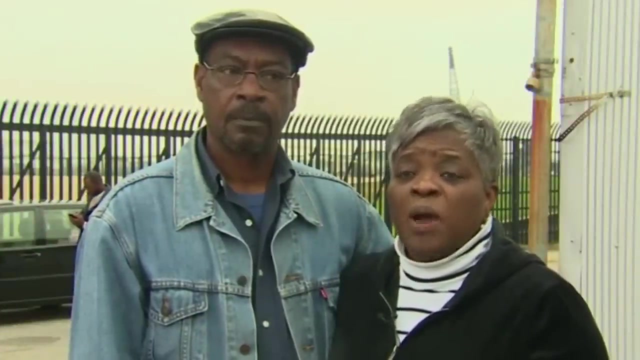 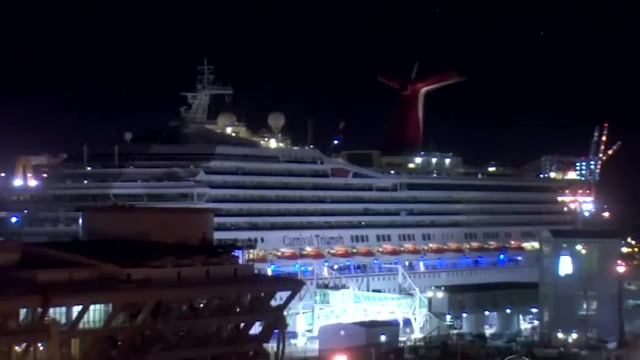 out of the ship In Mobile, worried family and friends gathered at the port anxiously awaiting the first glimpses of the Triumph and their loved ones. The Triumph was the largest cruise ship ever to dock at Mobile, and its final leg into the port required more than six grueling hours of work. 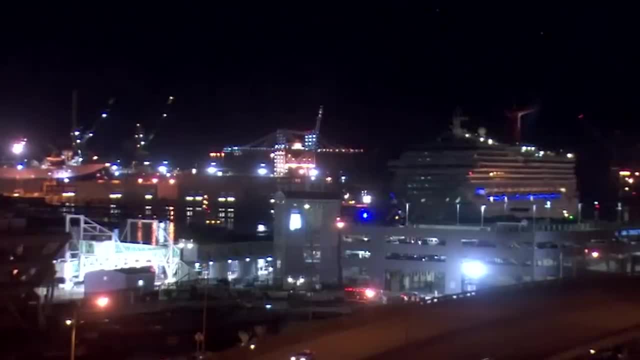 The Triumph was the largest cruise ship ever to dock at Mobile, and its final leg into the port required more than six grueling hours of work. The Triumph was the largest cruise ship ever to dock at Mobile, and its final leg in the port required more than six grueling hours of work. The Triumph was the last trick boat walking across the channel just established by Ark to ship from the St Malo vessel to the general fleet at Al McAnary port of YouTube. Both Gull table, Speakon Island, Bury and Dunke were in action eight hours before. 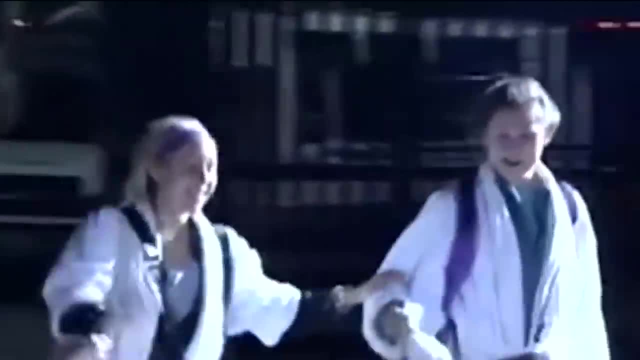 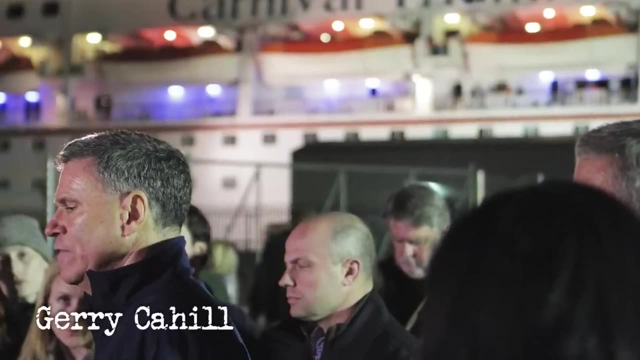 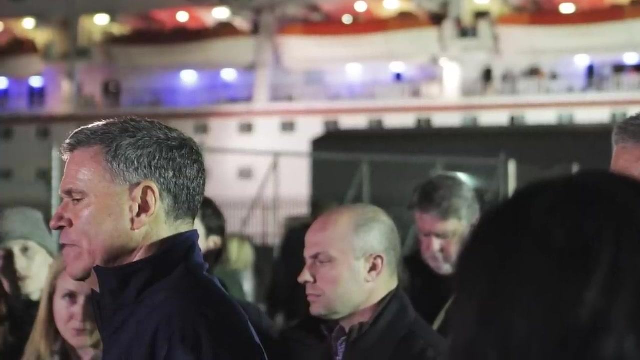 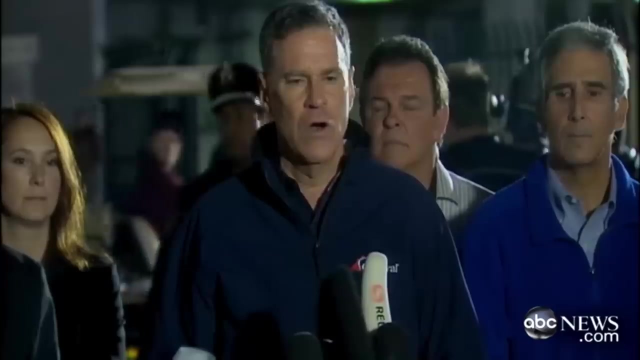 the Comforted at reasonable intervals, given the limited capacity to transport heavy cargo and things like Gull from the passengersl ouvert port arrangements. Read on for more information. the conditions on board were very poor. i know it was very difficult and i want to apologize again. 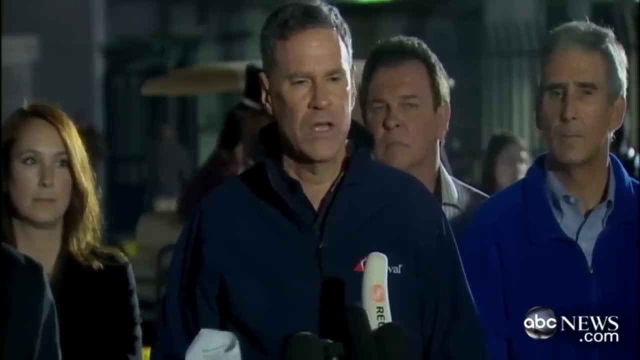 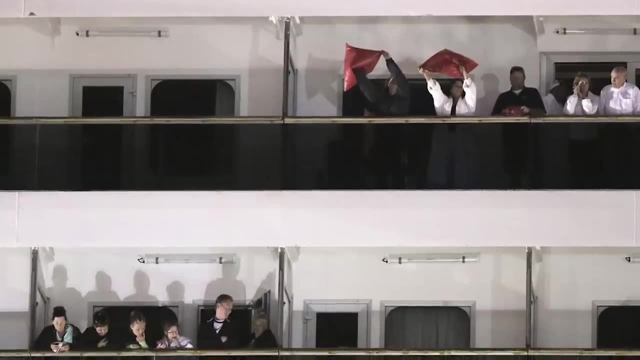 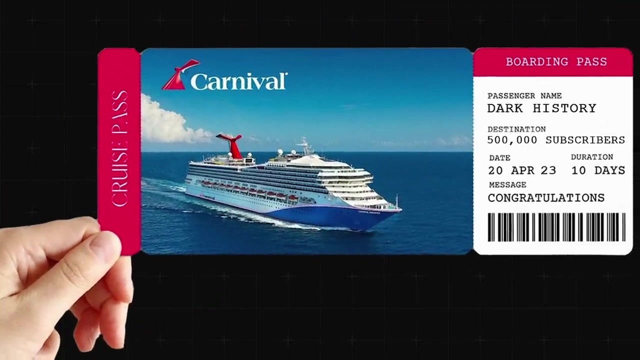 for subjecting our guests to that. we pride ourselves in providing our guests with a great vacation experience and clearly we failed in this particular case. but there was still more trouble in store for the passengers. in the carnival tickets small print, the cruise line added a protection clause if the performance of the proposed voyage is hindered or prevented by 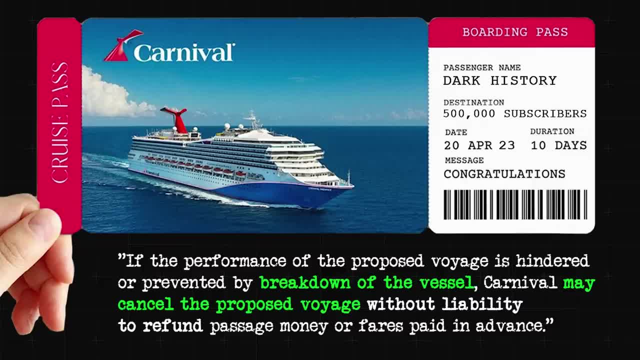 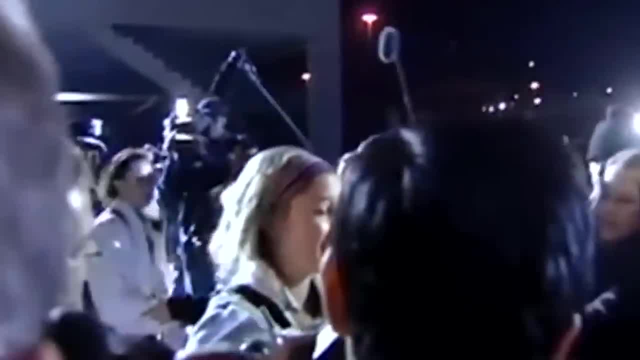 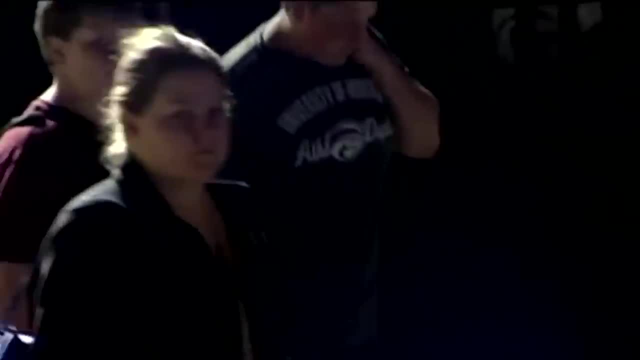 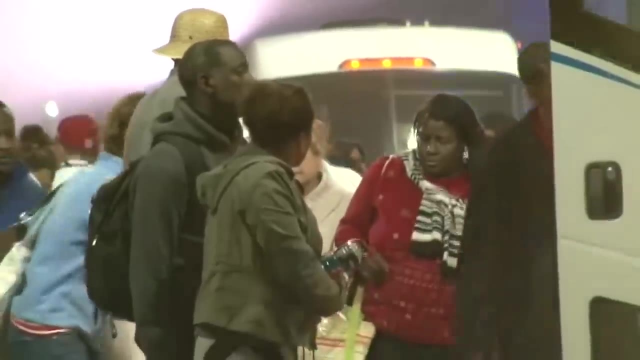 breakdown of the vessel, carnival may cancel the proposed voyage without liability to refund passage money or fares paid in advance. despite this, each passenger received five hundred dollars, a free flight home, a full refund for their trip and reimbursed most expenses on board, as well as a full credit for another cruise. this didn't stop passengers from filing a slew of lawsuits within. 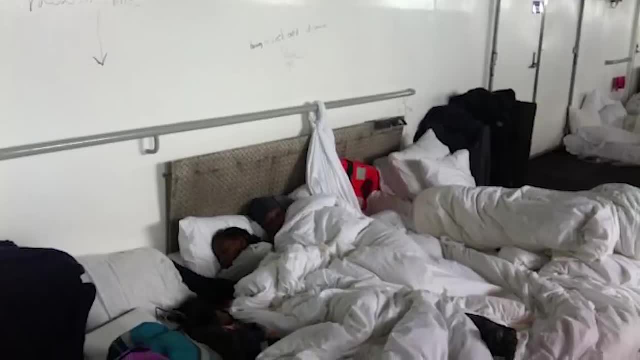 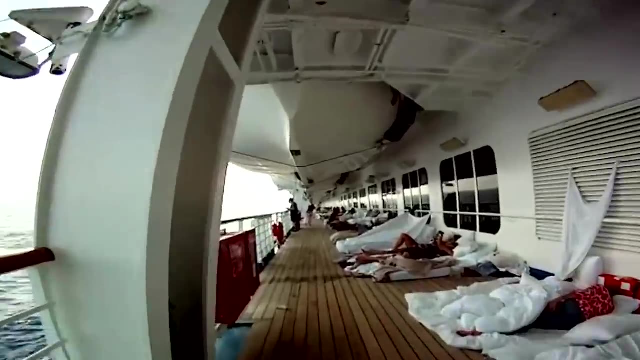 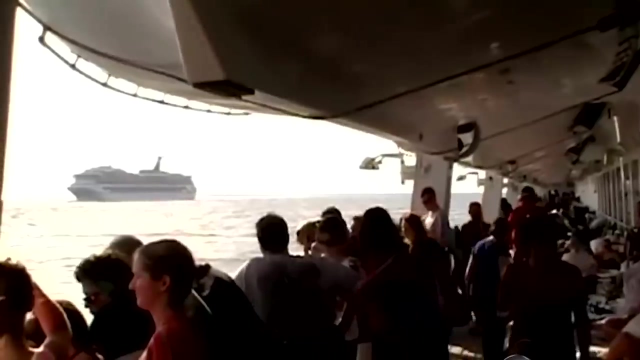 hours of reaching land. however, their chances of claiming compensation were slim to none, unless they suffered a personal injury. carnival ended up awarding one hundred eighteen thousand five hundred dollars in damages to twenty seven passengers, for doctors and hospital costs related to the ill-fated cruise, but the ship's woes continued while it was moored for.